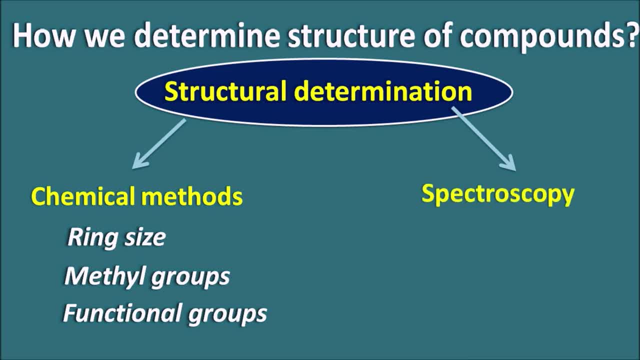 techniques, and particularly, we can use the spectroscopy in order to identify the structure, as well as to assess the structural features of the unknown compounds. For example, we can use the NMR spectroscopy, which gives the structural information and it acts like a fingerprint spectra. 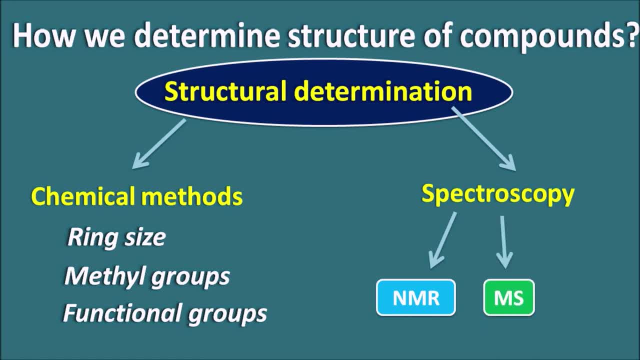 And we can also use the mass spectroscopy, where this technique will give the fragmentation pattern of an unknown compound, and we can also use the IR spectroscopy, which is again giving the fingerprint spectra of every unknown compound which can be matched with the already well known compounds. 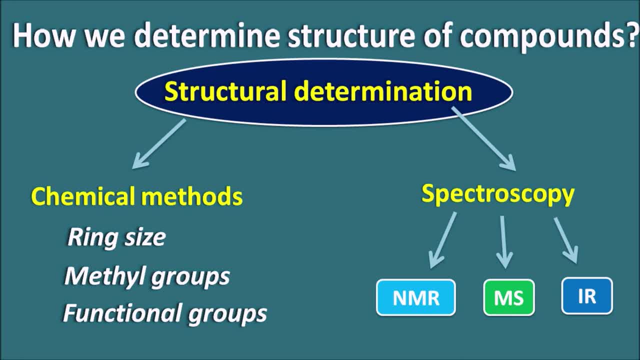 So in this way we can use any of these spectral techniques in order to assess the structure of the unknown compounds. but here we will see how we are going to use the mass spectroscopy where we can use the rule of 13.. So, role of mass spectroscopy in the structural determination. 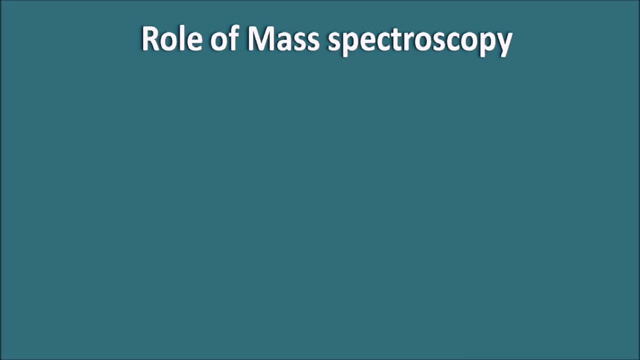 So what is mass spectroscopy? The mass spectroscopy involves the simple fragmentation of an unknown compound into the different types of fragment ions, and we can assess how many types of ions are going to be produced within the mass spectroscopy. For example, if an unknown compound is having a molecular weight of M, then it is undergoing. 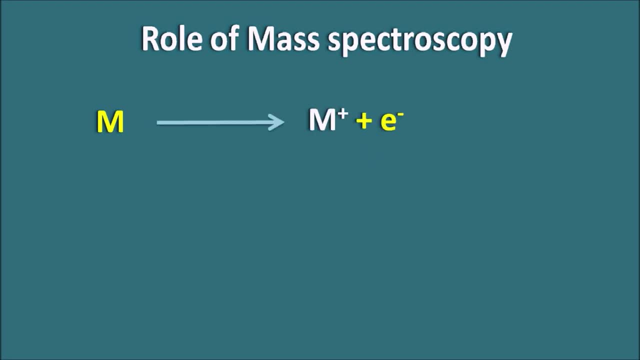 the ionization so that it is going to give the molecular ion M plus plus 1 LL. But this molecular ion is having some energy, so it cannot be stable and it can undergo the further fragmentation such that it is coming to a fragment ion M1 plus and M2, which 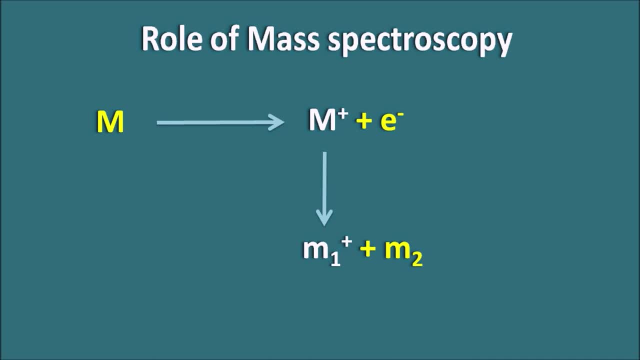 is a neutral fragment. In this way fragmentation can be continued until the stable fragment ion is going to be produced. So here in the mass spectroscopy the detector will detect how many types of ions are going to be produced and what is their M by Z ratio, where M is the molecular weight. 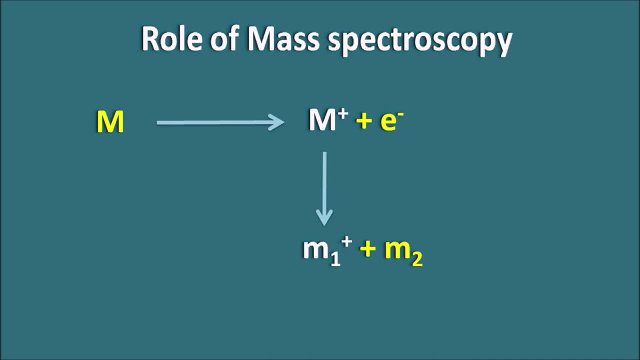 And Z is the valency of the ions. So Z is the valency of the ion. that means it is the positive charge of the ion, But here most of the times we focus on the univalent ions. so M by Z simply indicates the molecular weight where Z is equal to 1.. 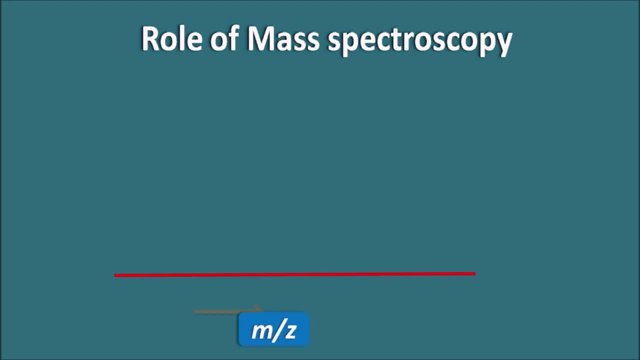 For example, let us take the mass spectroscopy of an unknown compound. So here, the X axis is the M by Z ratio, which simply indicates the molecular weight of the different types of fragment ions, And Y axis is nothing but the abundance, The relative abundance, of the ions that is going to be produced within the mass spectra. 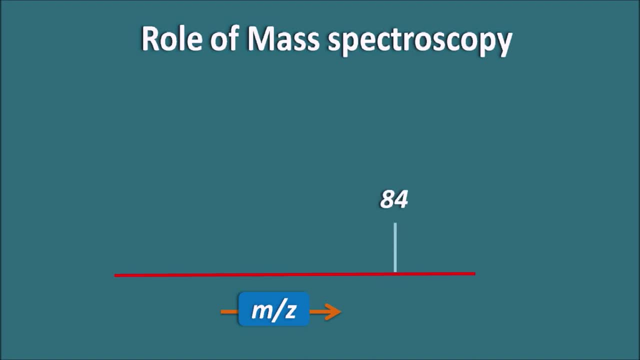 For example, for an unknown compound we got the one of the peak with M by Z ratio- 84. that means it is having a molecular weight of 84, and another peak is at the 55 and we have seen the few of the other peaks like this. 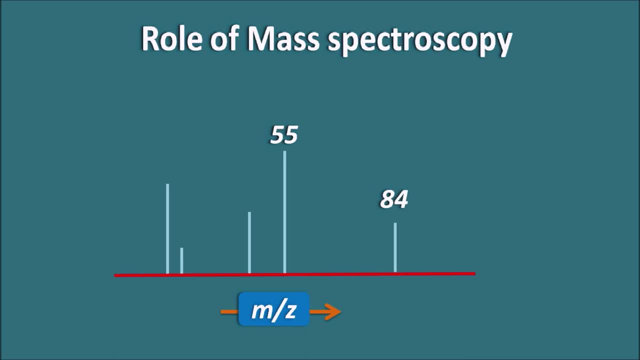 Now here, what is the peak? corresponding to 84 indicates. So what are the peak which is going to lie at the right side of this mass spectra? mostly it indicates the molecular ion peak. So this is the peak, And we can also sometimes observe few of the quasi-molecular ion peaks which are greater. 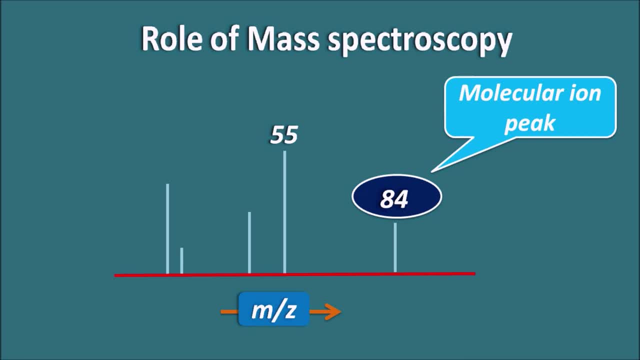 than this molecular ion peak. but these peaks will have less intensity, so they will have the less height. so we can easily detect which is the molecular ion peak. So for this example 84 indicates a molecular ion peak. And here, in this mass spectra of this unknown compound, we can observe a tallest peak which 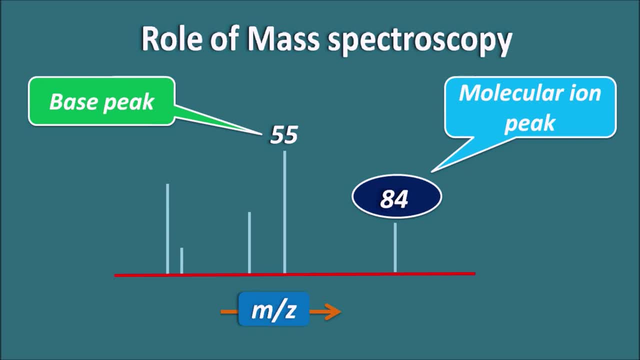 is called as the base peak. that means the molecule is undergoing a fragmentation to give a stable fragmentation. So we can see that it is having a particularEREX or a fragment ion which is having a molecular weight of 55. Now, by knowing this molecular spectra of an unknown compound, we know the different molecular 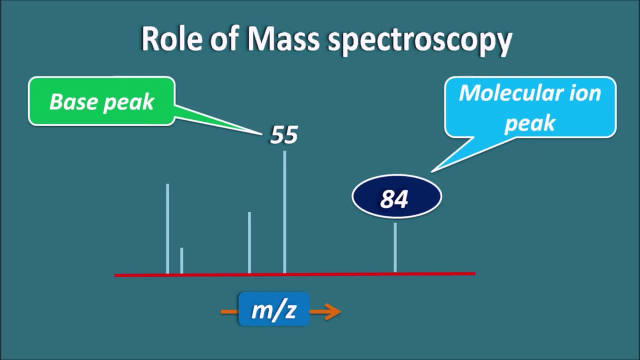 weights of ions produced in the molecular spectra and from this we can assess the structural features of unknown compound. For example, here, what is the molecular ion peak is the 84, and we can calculate the index of hydrogen deficiency by using the rule of 13.. 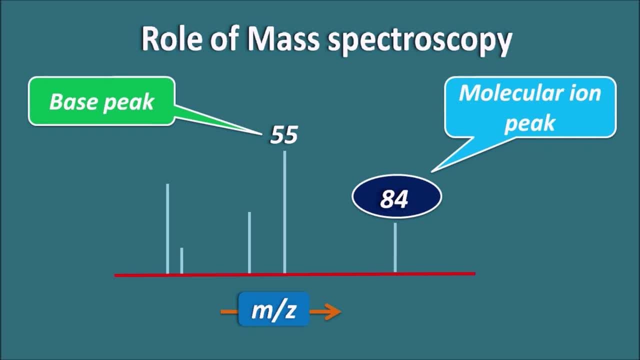 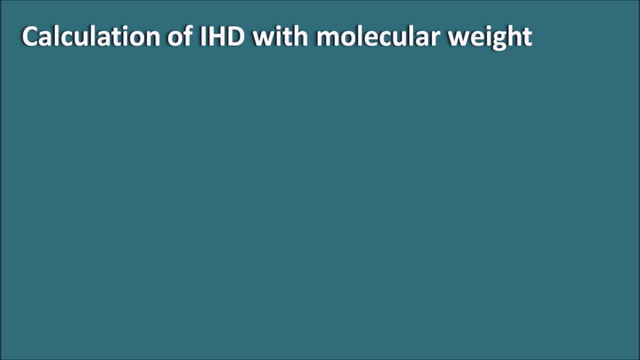 So the one that we can calculate the index of hydrogen deficiency by using the rule of 13. be the possible structural features of this unknown compound. Now let us see the calculation of IHD with the molecular weight. So, whenever the molecular weight is known by the mass spectroscopy, we can apply the 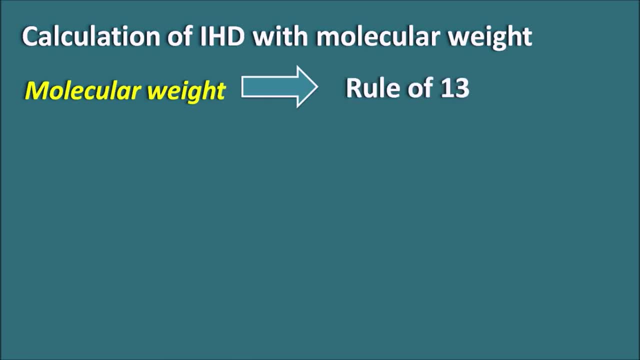 rule of 13 in order to assess the IHD value of the unknown compound. The rule of 13 is a simple calculation where we have to divide the molecular weight by 13 and when we are going to divide, we will get the quotient as well as the remainder. 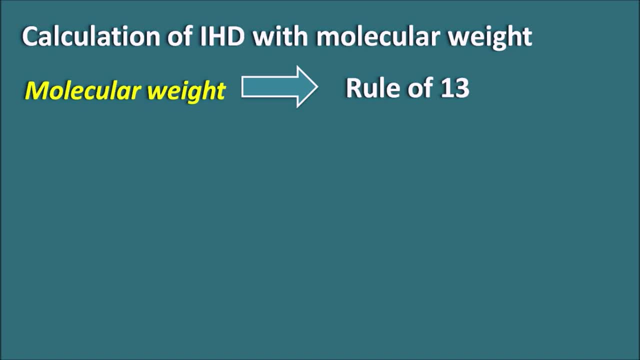 The quotient can be represented as the N value and remainder as the R value. Then we can write the molecular weight as N and R by 13.. So this is nothing but N plus R by 13, where N is the quotient and R is the remainder. 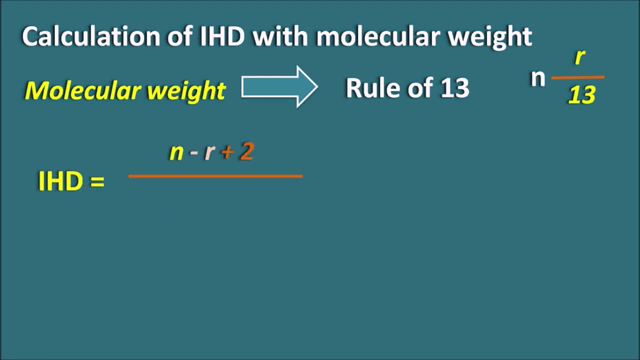 Then we can calculate the IHD value, as IHD is equal to N minus R plus 2 by 2.. So let us take one example here. Let us take the first example, cyclohexane. Now let us calculate the IHD value by all the measurements. 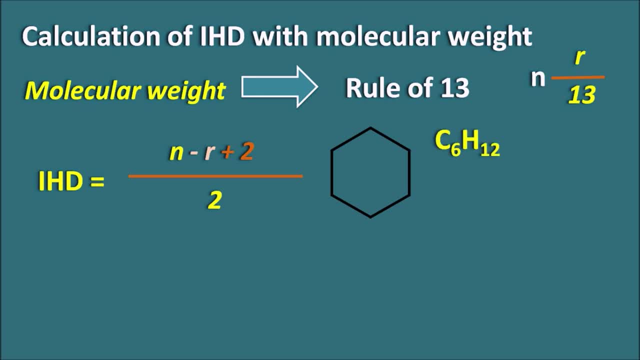 So this is the cyclohexane having the molecular formula C6H12.. And if we compare with the standard molecular formula, it will be C6H14.. So the number of hydrogens less is the 2.. So IHD value will be 2 by 2, that is equal to 1.. 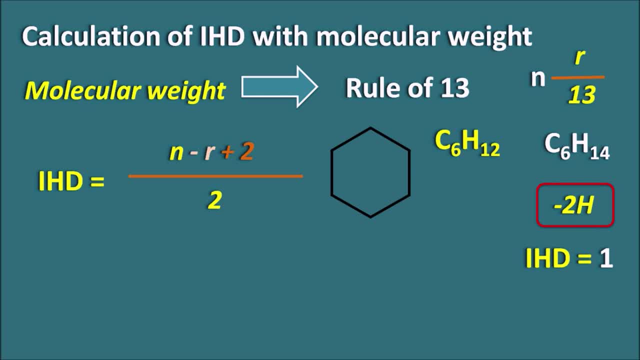 So cyclohexane is having the IHD value as 1.. And again we can see by structure: it is having one cyclic ring without any pi bond. So IHD value is again 1.. And now let us check by the molecular weight. 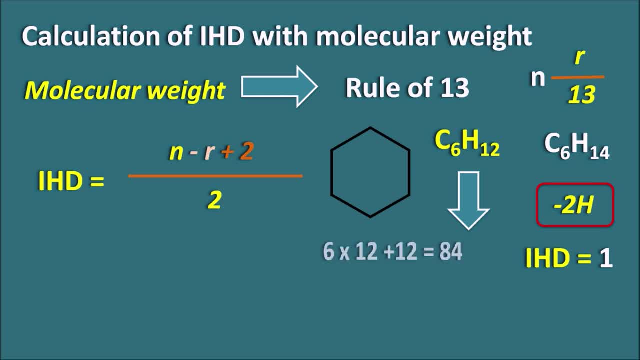 The molecular weight of this cyclohexane is 6 into 12, because carbon is having the atomic weight as 12 and hydrogens are having the atomic weight as 1.. So 6 into 12 plus 12, which gives the 84.. 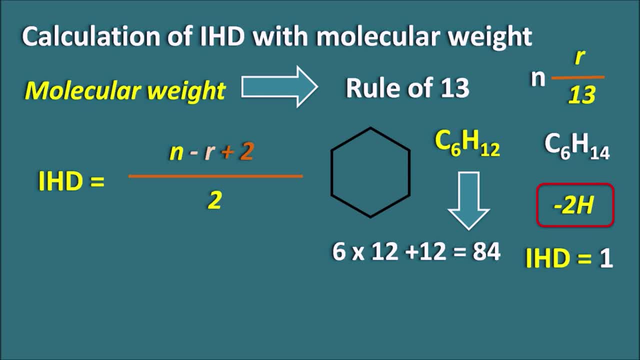 Now let us divide this 84 by 13. So when we divide by 13,, we will get the 13 into 6 plus 6, which can be written as 6 and 6 by 13. So 13 into 6 is nothing but 78 plus 6 is nothing but 84.. 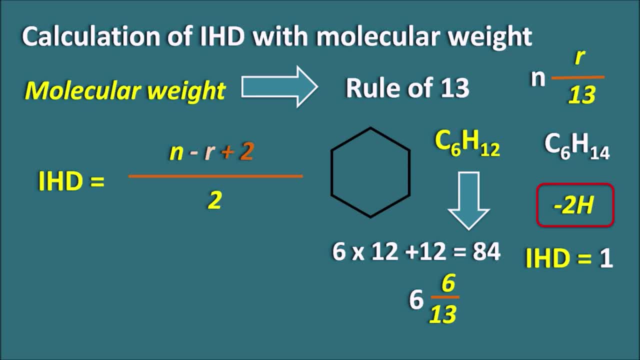 So this is the cyclohexane. So this is the cyclohexane. So this is the cyclohexane. So the cyclohexane is less than or equal to 84.. So this can be written as 6 and 6 by 13.. 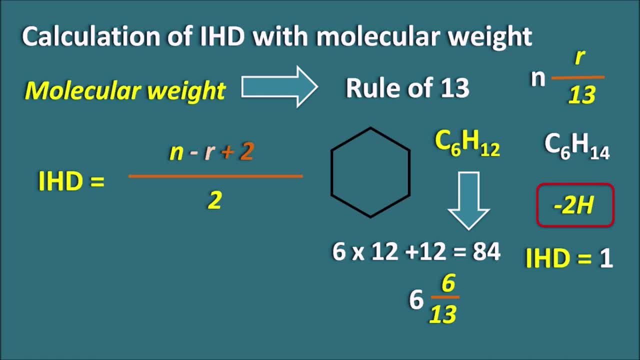 So now here, the quotient n is the 6 and raminder r is again 6.. So if we calculate the IHD value, the IHD is equal to 6 minus 6 plus 2 by 2, which gives the 1 value as the IHD. 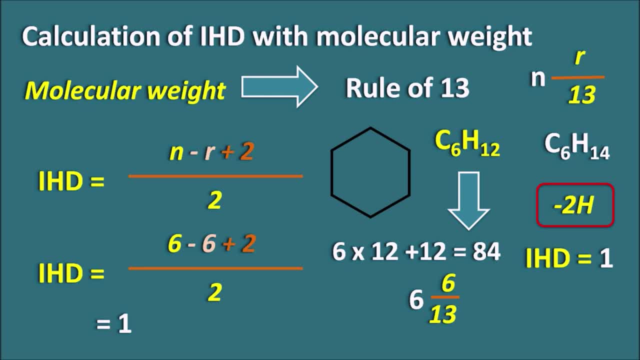 So now we can easily check that if we calculate the IHD value by seeing the structure or by seeing the molecular formula or by taking the molecular weight, We will get the disastrous THE the same value. But which formula should be used it depends on the data we have, Suppose we have. 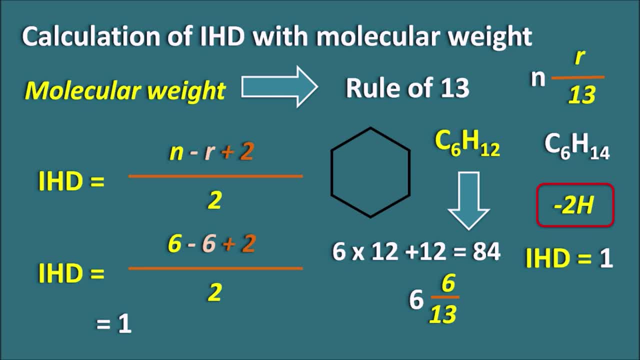 the structure of the compound, we can check the number of cyclic rings and the pi bonds so that we can get the IHD value directly. Otherwise, if we have the molecular formula, we can compare the molecular formula with a saturated open chain compound and we can see the number of hydrogens. 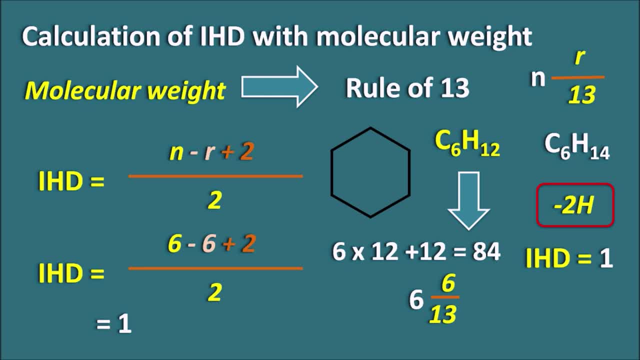 that are less and when we divide this value by 2 we will get the IHD value. But whenever the molecule is having the heteroatoms, we have to use the corrected molecular formula. Whenever the molecular weight is given, we have to apply the rule of 13 and we have to divide the molecular 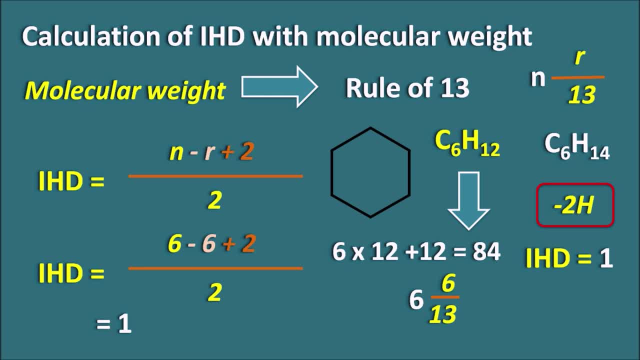 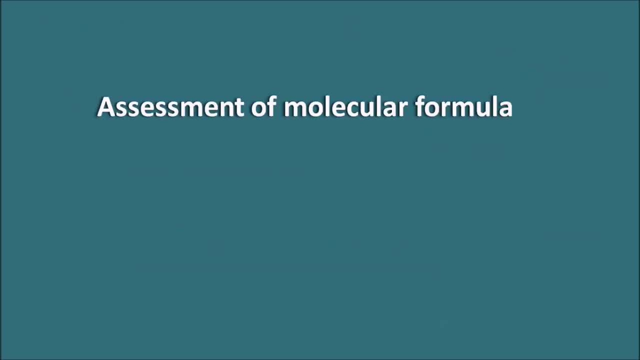 weight by 13, so that we have to use the quotient and reminder to calculate the IHD value with the formula n minus r plus 2 by 2.. Now let us see the assessment of molecular formula of unknown compound by using rule of 13.. So molecular weight is given as 84 for this example. 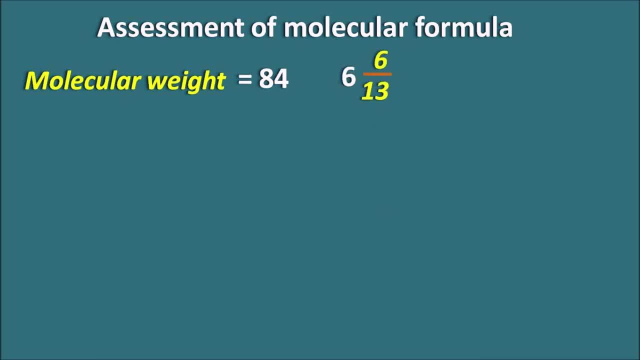 By applying this rule of 13, we can write the 84 as 6 and 6 by 13. So here the quotient is 6 as well as the reminder is 6.. For this unknown compound, we can write the molecular formula as Cn, Hn plus r. 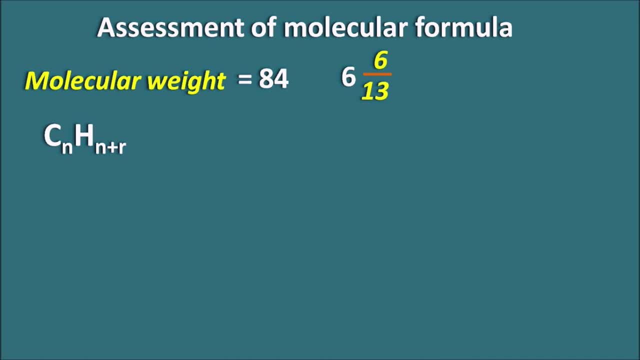 where n is the quotient and r is the reminder. So for this compound the molecular formula will be C6 H 6 plus 6, because n is equal to 6 as well as r is equal to 6.. So this is nothing but C6 H2.. 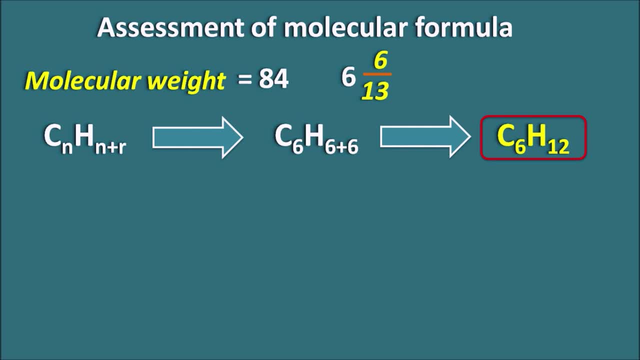 So the unknown compound is having a molecular formula C6, H12, whose molecular weight is 84. So when we know the molecular weight of this unknown compound, we can easily write its molecular formula by using the rule of 13.. And suppose if the compound is having a heteroatom like: 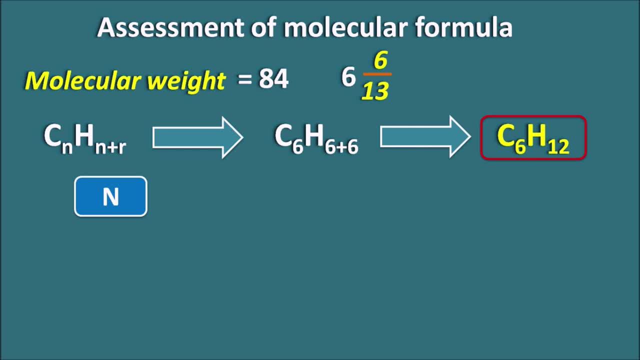 the nitrogen, then what will be the molecular formula? Because nitrogen is having an atomic weight of 14. so in order to add the nitrogen we have to deduct C? H2, because carbon is 12 and hydrogen is 2. So total is 14.. So we can add the nitrogen and we can deduct the C? H2 from this molecular formula. 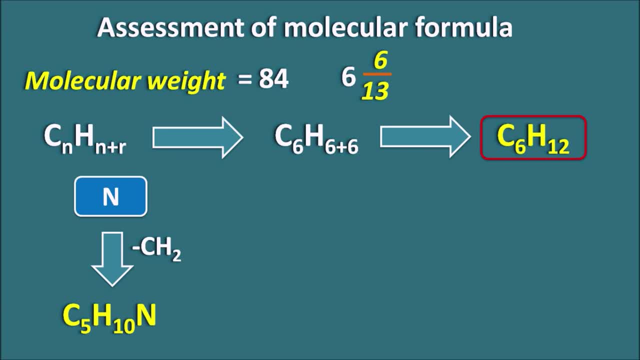 So it will be C5 H10 n. So from C6 H12 we have deducted 1 carbon and 2 hydrogens and we have added 1 nitrogen, So the molecular formula will be C5 H10 n. Similarly, if we want to add the oxygen, 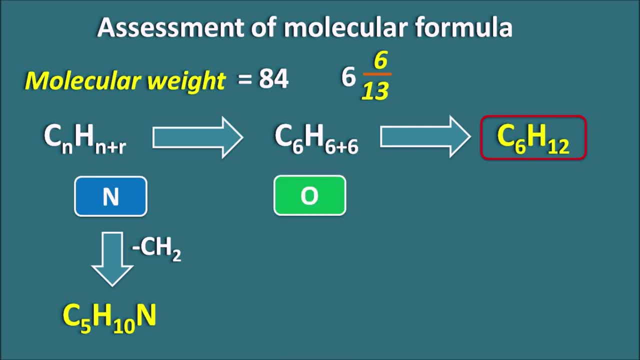 since oxygen is having the 16 atomic weight, then we can deduct the minus C, H4, because carbon is 12 and hydrogen is 4. So total is 16.. So then the molecular formula becomes C5, H8, O, And similarly, if we want to add 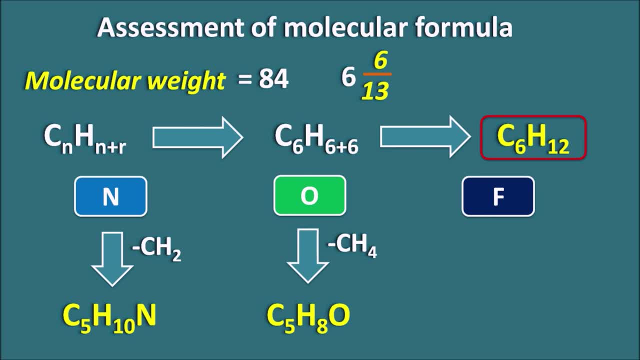 the fluorine Fluorine is having the 19. So we can deduct by 1 carbon and 7 hydrogens, So it becomes C5, H5, F. In this way we can write the possible molecular formulas for the unknown compound, if we know its molecular weight, by applying the rule of 13. And we can 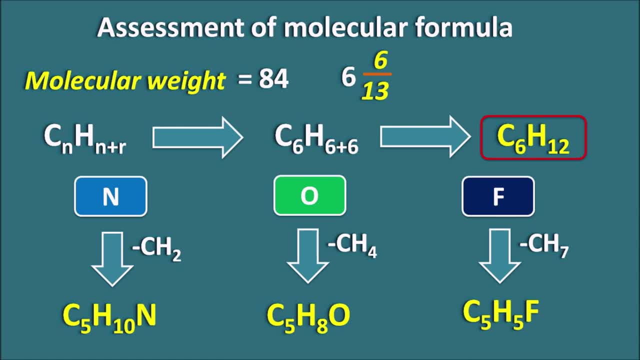 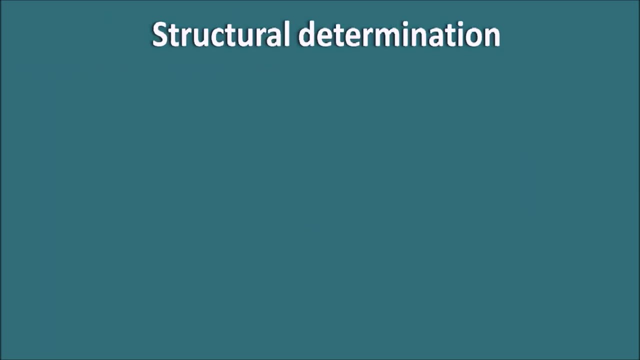 also assess whether The compound is having the nitrogen oxygen, fluorine or any other atoms by again seeing the spectral features as well as by using some chemical methods. So by combining all the data we can determine the possible structure for an unknown compound. Now let us see the structural determination. 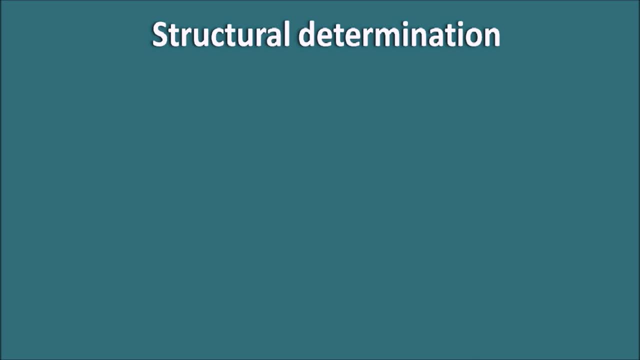 of the unknown compound with the use of its molecular formula as well as the IHD values. Suppose, if the molecule is not having any heteroatom, then for the molecule having a molecular weight 84. The molecular formula will be C6- H12, and for that we can write the different structures like this: 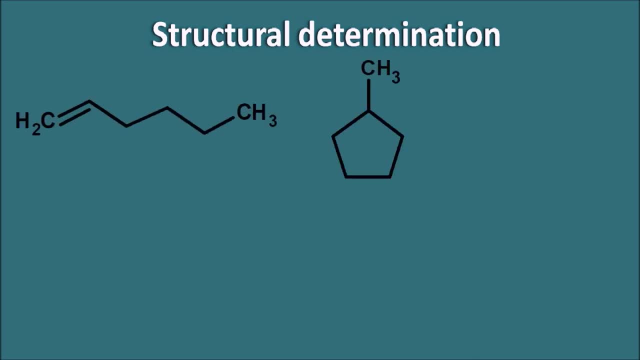 So one of the structure is 1 hexene, and another structure is methylcyclopentane, and another one is the ethylcyclobutane, and another one is the cyclohexane. In this way we can write so many structures for a given molecular formula. So all we have seen this example in the our previous video. 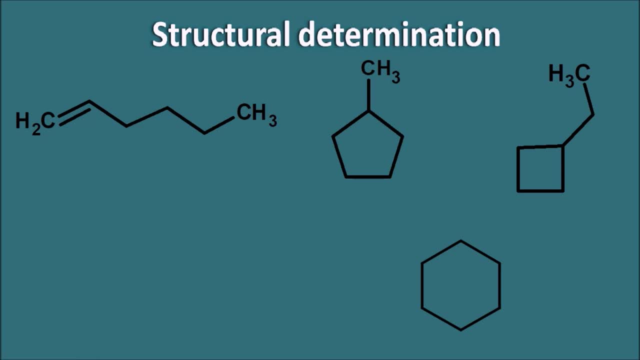 And here we can use this information along with the mass spectra and we can assess the possible structure for the unknown compound. For example, if the compound is having any cyclic structure like the cyclopentane cyclobutane or cyclohexane, within the mass spectra it will give a peak like 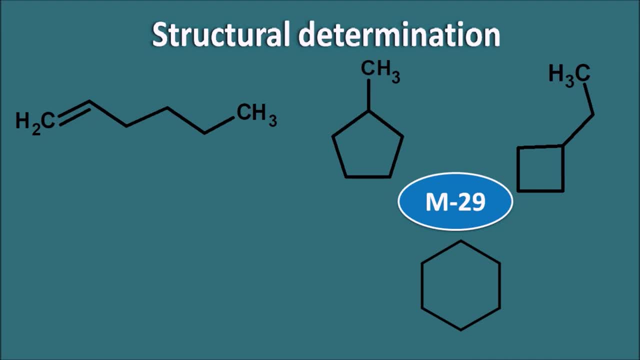 M-29, where M is the molecular weight. So if the molecular weight is 84,, 84-29, that becomes 55. So it will give a peak at the 55. Similarly, if the molecule is a alkene, again it can give the peak at. 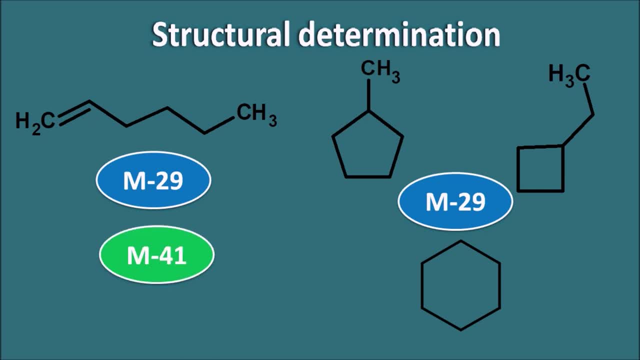 the M-29. along with this peak It will also give another peak at the M-41.. So if both of these peaks are present, then we can say that it may be a alkene. Cycloalkenes also give the M-41 peak. but 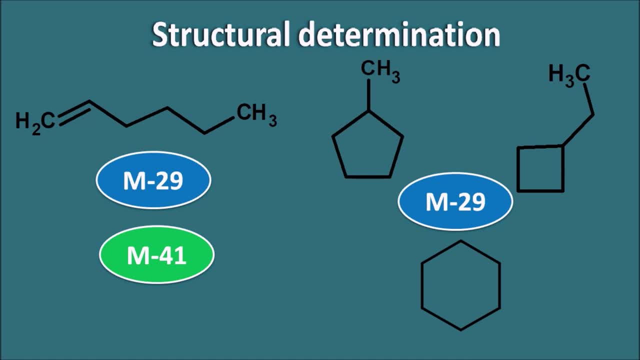 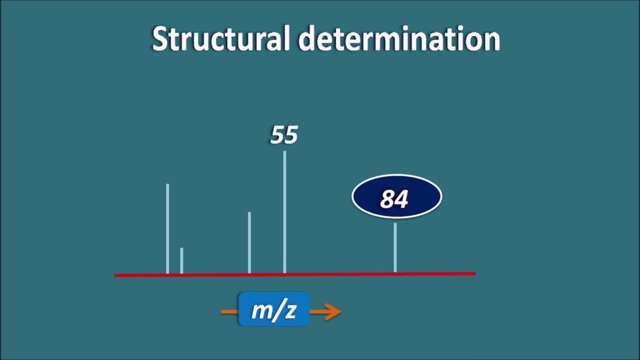 their abundance is very low compared with the alkenes. So just by seeing the type of peak, as well as its relative abundance, we can assess what may be the structural feature of the unknown compounds. Now, if we go to the previous example, we got the mass spectra like this. So here the 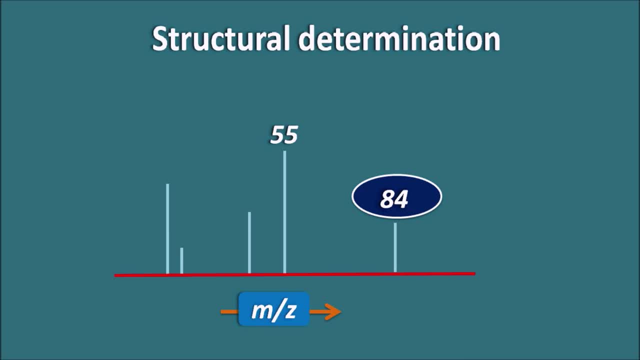 84 is the molecular ion peak. and what about the 55?? So this 55 indicates simply M-29.. M molecular weight is 84, then M-29 will be 55. So here this spectra indicates a peak corresponding to M-29.. So it may be a cycloalkene, or it may be alkene, And here suppose we got another peak at. 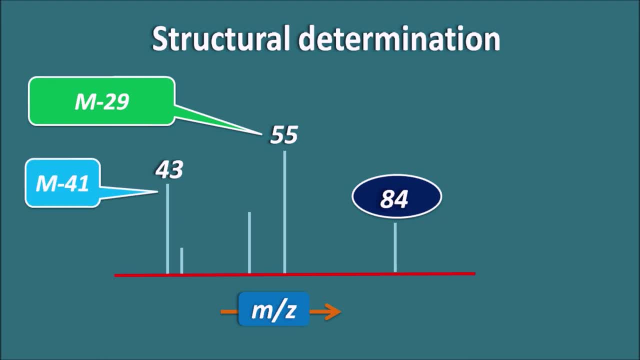 43. What this 43 peak indicates, So 43 is simply M-41. And we can also see that the abundance is significant in this spectra. That means it may be an alkene. it may be 1-hexene, 2-hexene, 3-hexene. 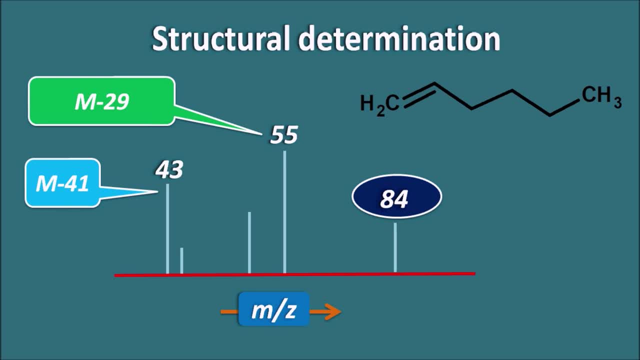 whatever may be, That means we can say that it is having an alkene in this compound because it is giving a M-41 peak with some significant abundance, And again we can confirm this by using the IHD value. So for this compound the IHD value should. 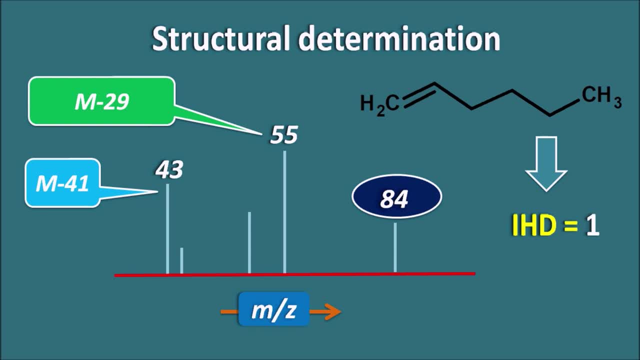 be 1 because it is having 1-pi bond. and already we have calculated the IHD value by use of rule of 13, where we got the IHD value as 1 for the molecule with molecular weight 84. So in this way, by using the mass spectroscopy, we will get the different types of ions at 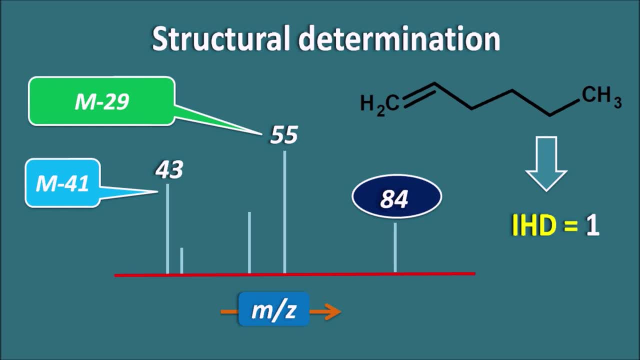 the different molecular weights and for each molecular weight we can assess the possible structure by using the rule of 13.. So rule of 13 can be used to determine the molecular formula of unknown compound, as well as it can also be used to identify the index of hydrogen deficiency. 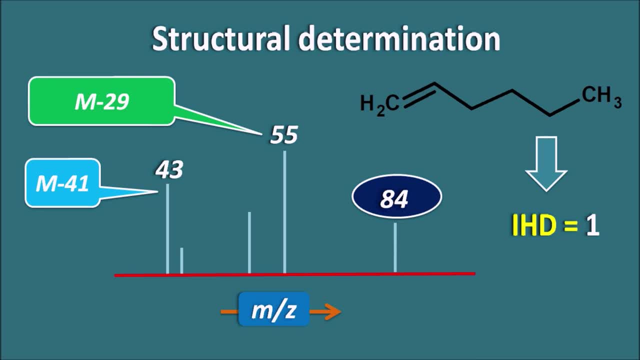 By combining all these we can assess the possible structures for each type of fragment ion. By combining all these data, we can assess the structure of the unknown compound. So that is the use of the rule of 13 in this mass spectroscopy. So rule of 13 is a simple way of calculation of molecular formula, where we have to divide. 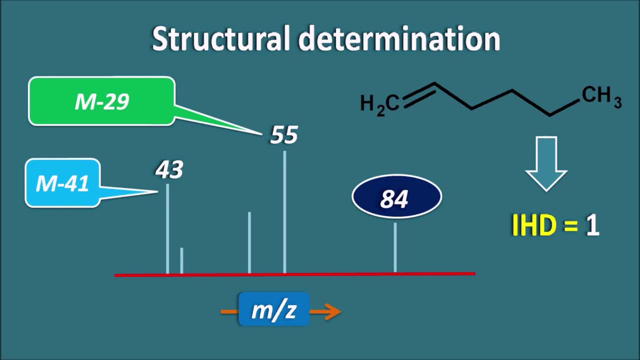 the molecular weight by 13.. And then the molecular formula. The molecular formula will be CnH, n plus r, where n is the quotient and r is the remainder. Similarly, the IHD value can be calculated as n minus r plus 2 by 2..